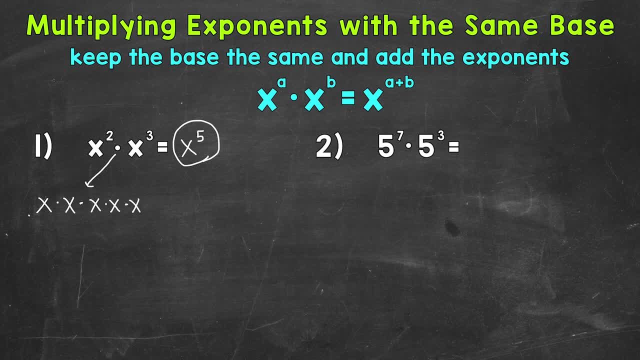 x times x. This right here, this is x squared, And this right here, this is x cubed. And you can see that we have 5 x's there, which is x to the power of 5.. Let's move on to number two, where we have 5 to the power of 7 times 5, cubed. 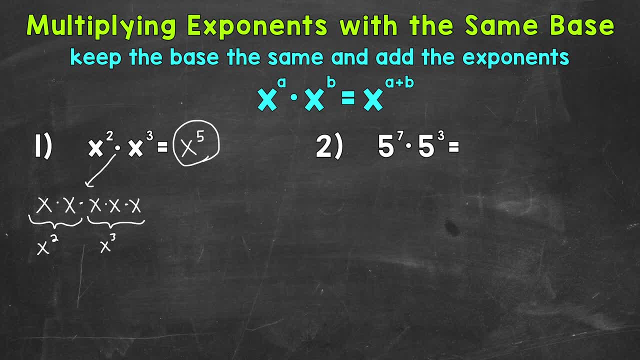 Well, keep the base the same. Our base is 5.. And then we add the exponents, So 7 plus 3 is 10.. So 5 to the 10th power, which equals 9,765,625.. 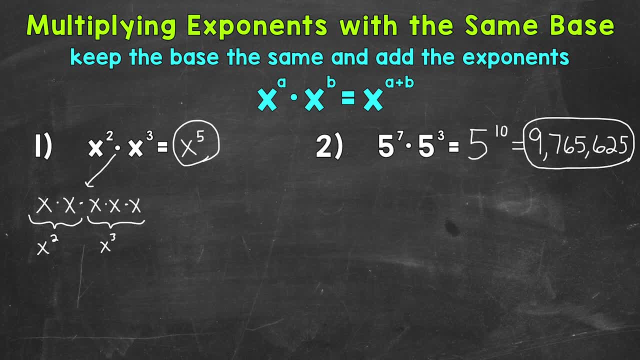 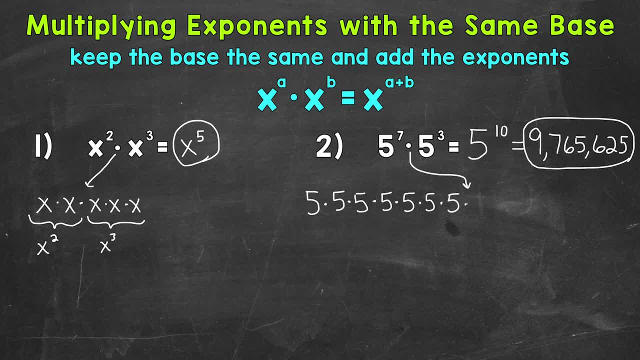 And then we bring our multiplication sign down in the middle here And then 5 cubed is 5 times 5 times 5.. So we have 5 to the power of 7. Represented right here. Then we have 5 cubed, represented right here. 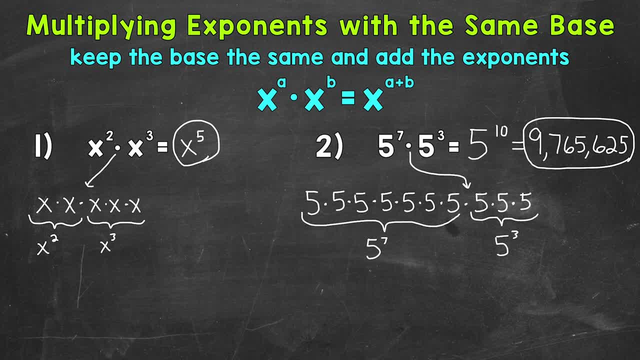 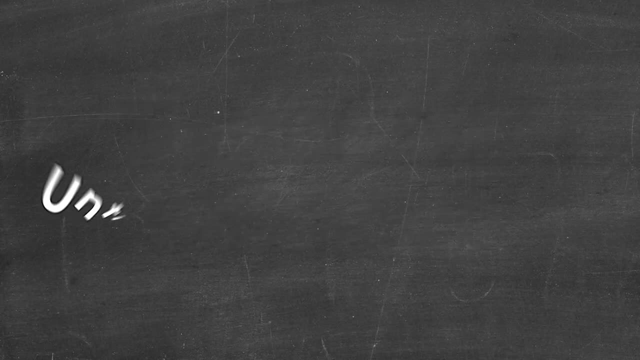 And that gives us 5 to the power of 10.. So remember, keep the base the same and then add the exponents when multiplying exponents with the same base. I hope that helped. Thanks so much for watching. Until next time, peace.